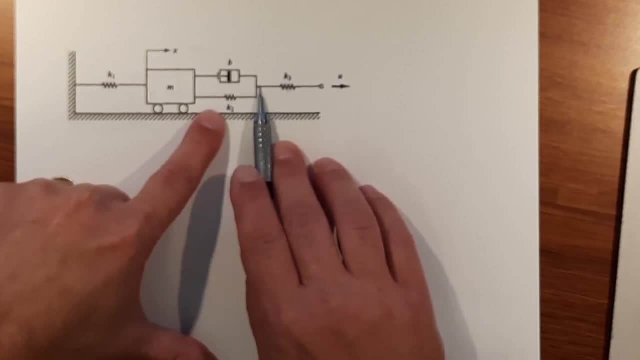 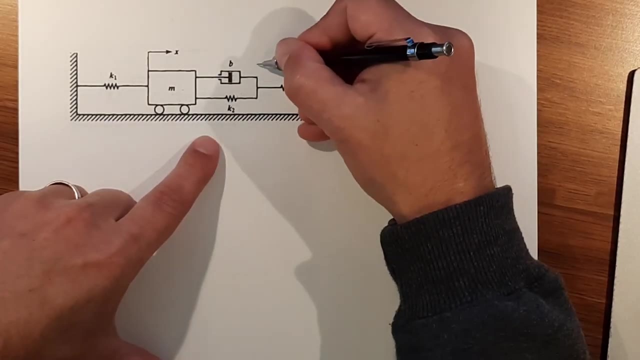 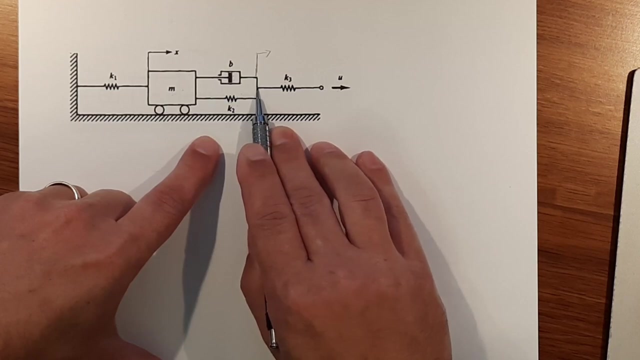 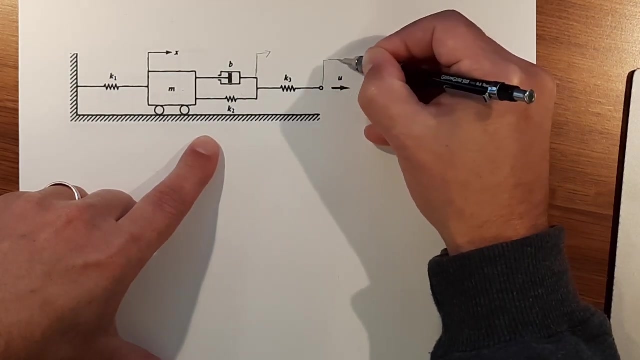 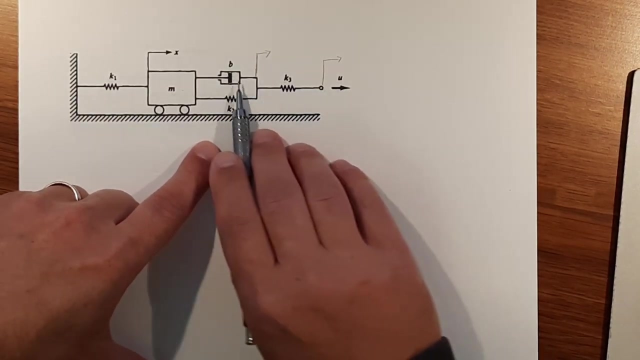 spring connected at a point that is connected to another spring and a dampener. So we can separate these and we can put a point here in between this spring and this pair of spring and dampener, and then we can have our point here at where U and K3 meet as another point, And we're 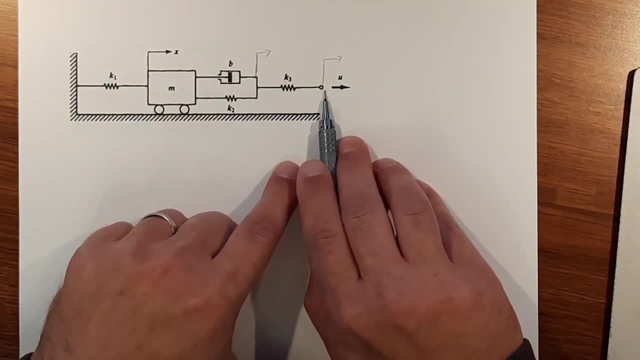 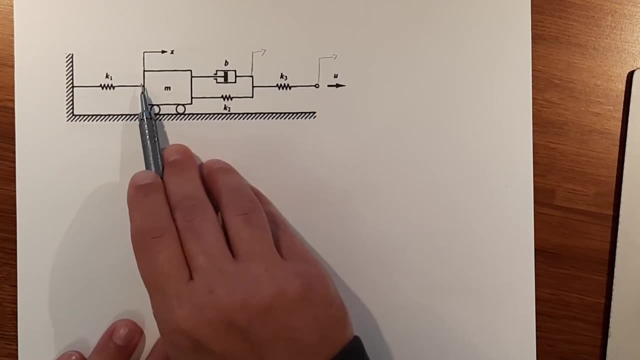 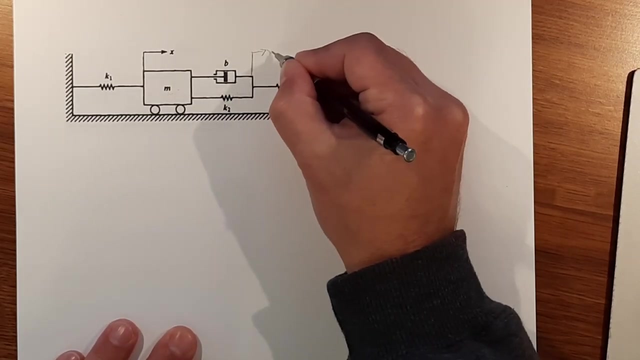 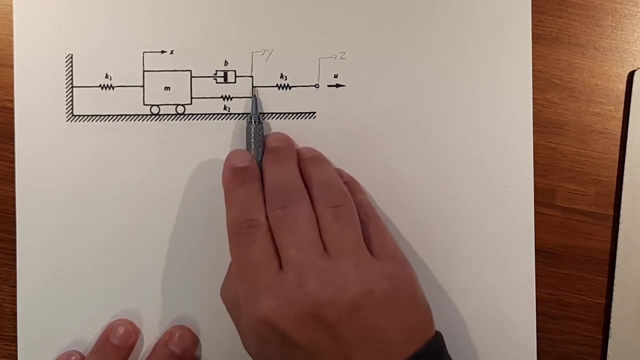 going to do this because we know that when we apply the force U, that each of these points are going to have a change in position that are different relative to our change of position on X, So point Z and point Y. So point Z can move more than point Y, which could. 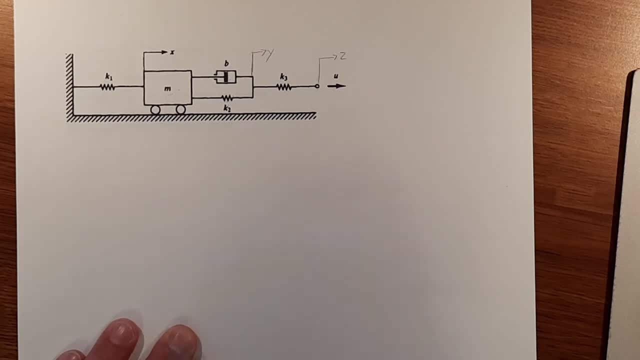 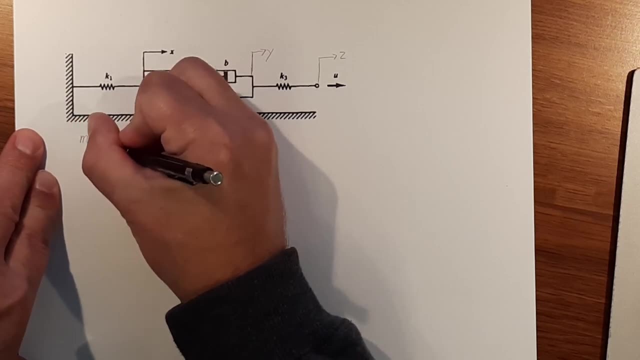 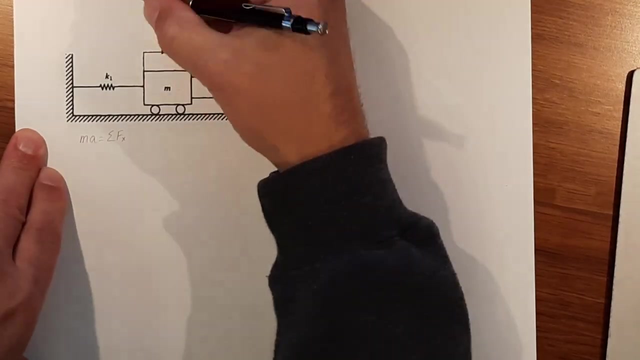 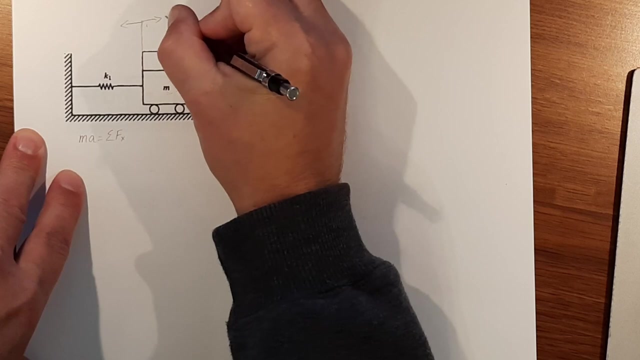 move more than point Z. So to start writing our differential equation, we can start off with mass times. acceleration equals the sum of forces in the X position. We're going to go ahead and label our directions. So we're going to have anything to the right is positive and anything to the left is going to be. 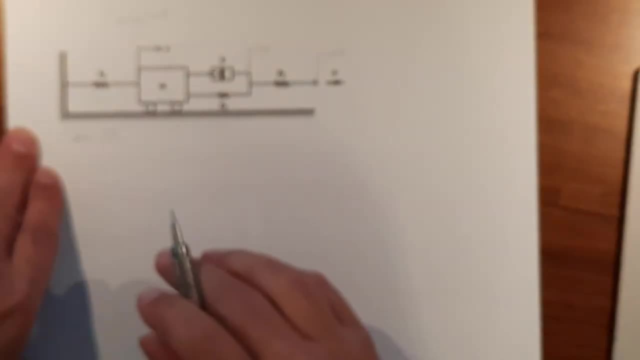 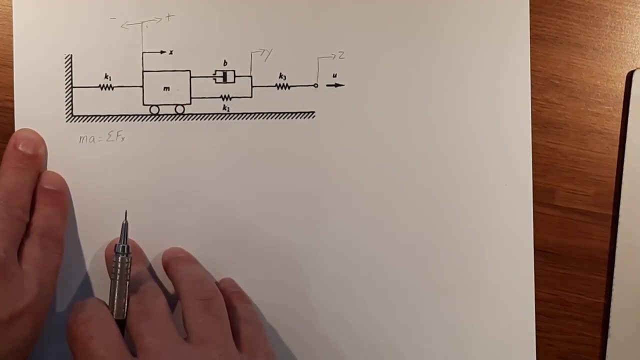 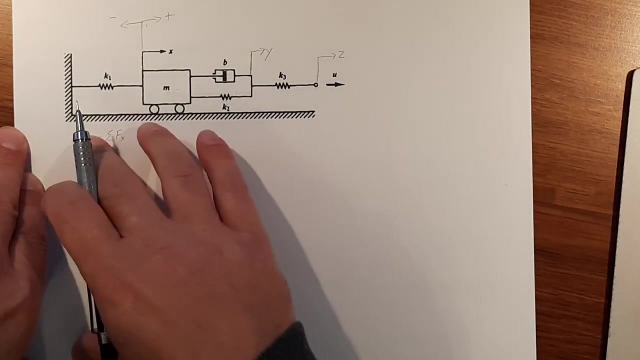 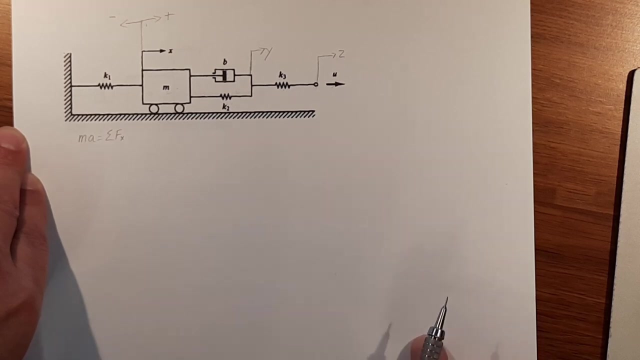 negative, And there's two different ways you can write this, depending on how you want to write the signs, And I'm going to write them both ways, so you can see that, even though they're different, they equal. they end up equal the same at the end. 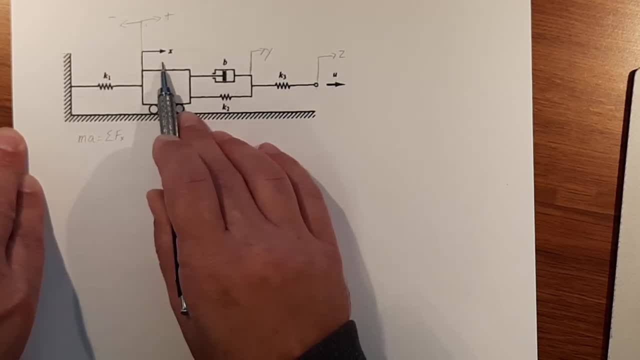 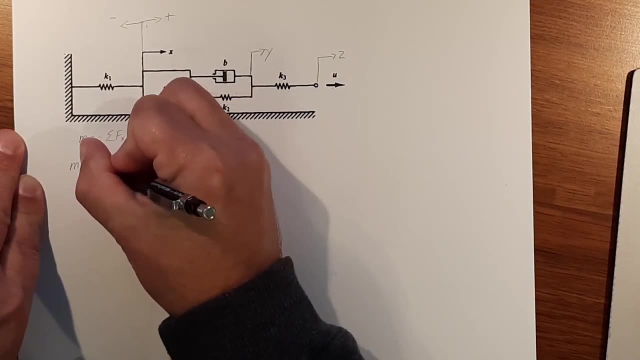 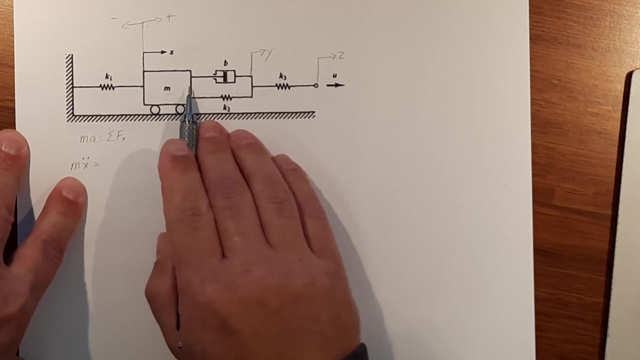 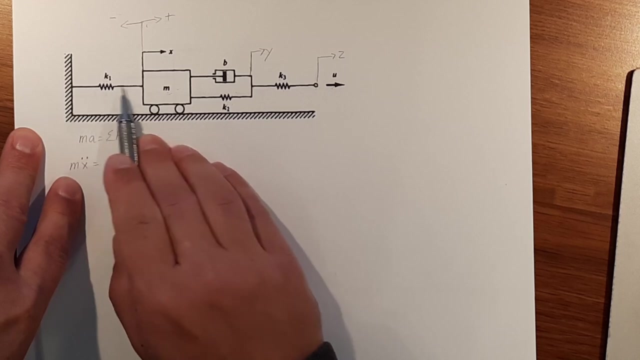 So let's start off with our mass here and our position X. so we have mass times acceleration. We're going to change that to x. double dot is equal to our sum of forces. So, starting on the left, we're going to have K1 and that is going to be. 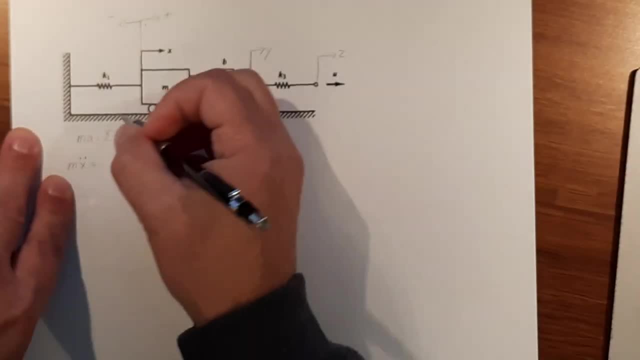 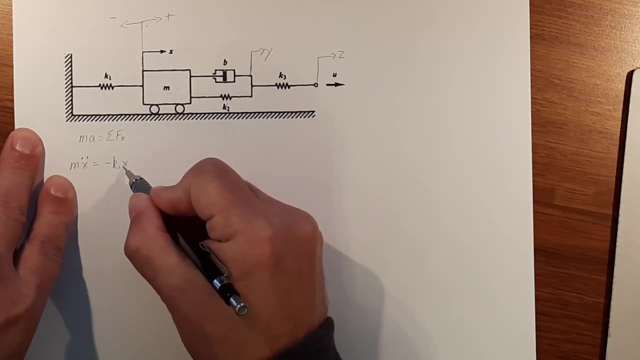 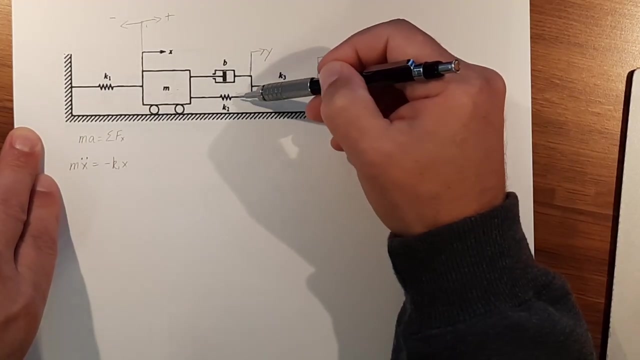 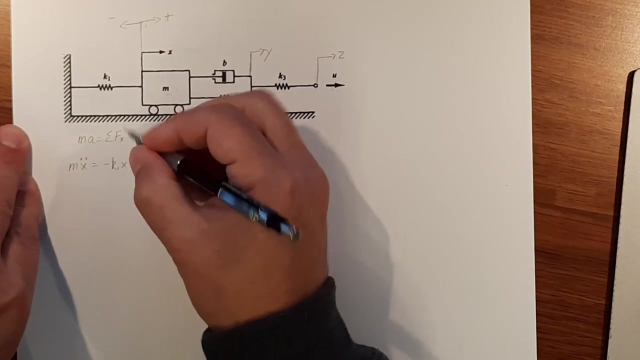 wanting to pull this mass to the left, So it's going to be a minus K1 times X times X. now, if we look to the right, we have a dampener and a spring, so we're going to break these up and account for them individually. so we're going to have 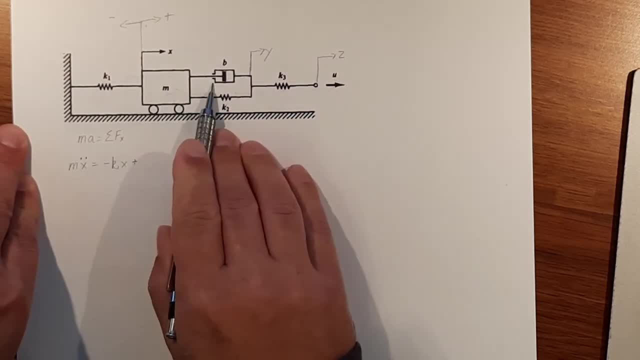 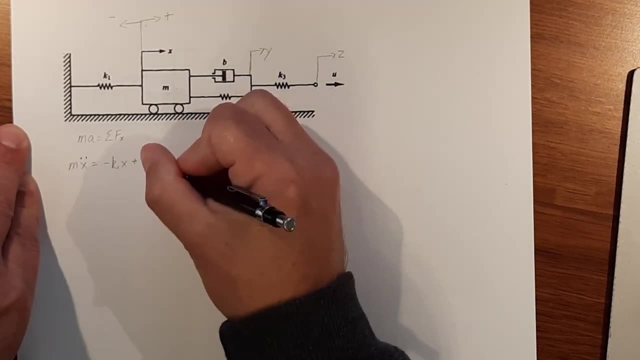 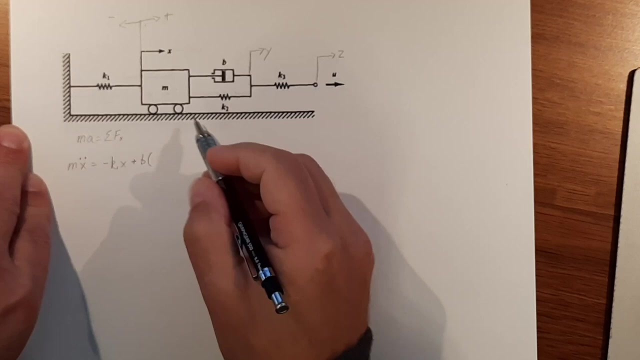 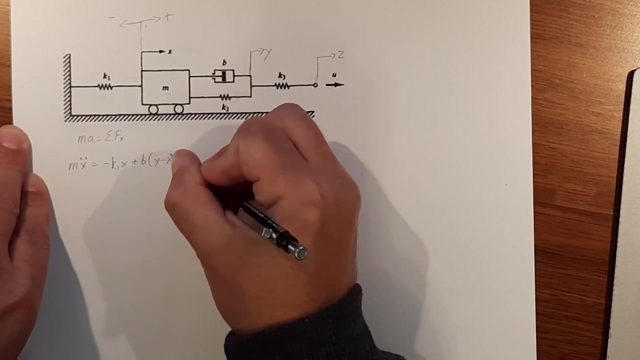 a plus because this dampener is going to pull this mass to the right B times its change in velocity. since dampener is effect of velocity, we're going to have Y, dot-X, dot. and now for the spring, since it's going to be a vellum now, we're going to have a plus because this dampener is. 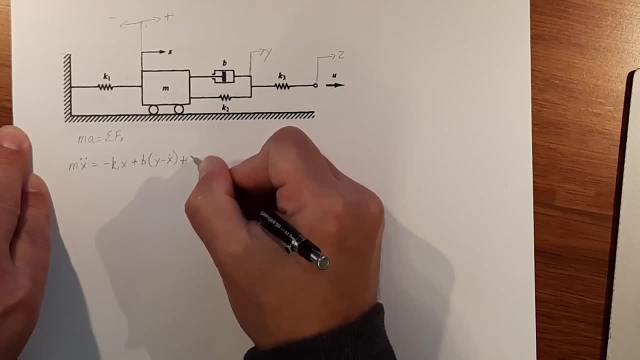 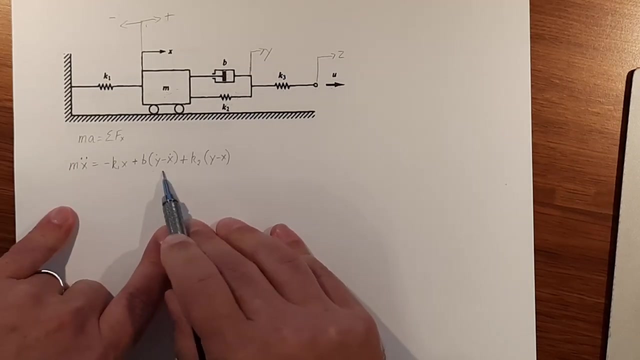 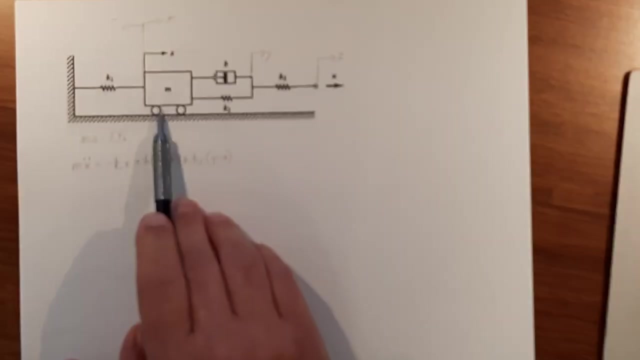 be wanting to pull this mass to the right, We're going to have plus k2 times its change in position, and this change in position is y minus x. Now we're not going to count for k3 in this equation, because k3 does not directly affect the change of position of our mass. So we're going to have 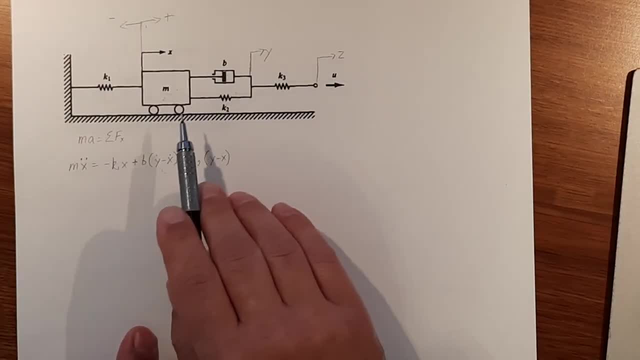 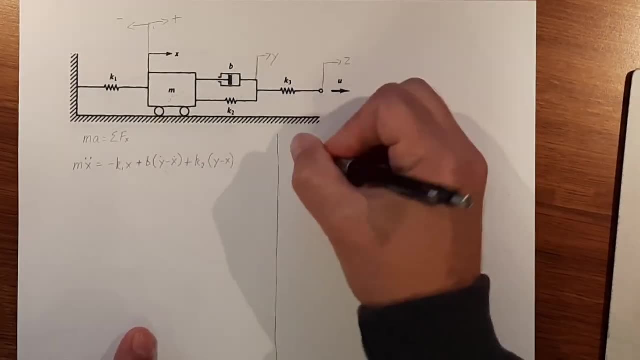 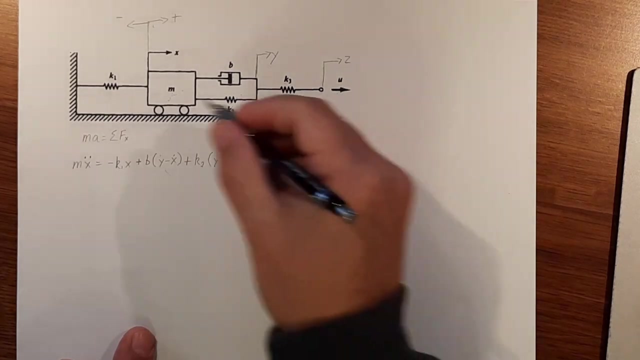 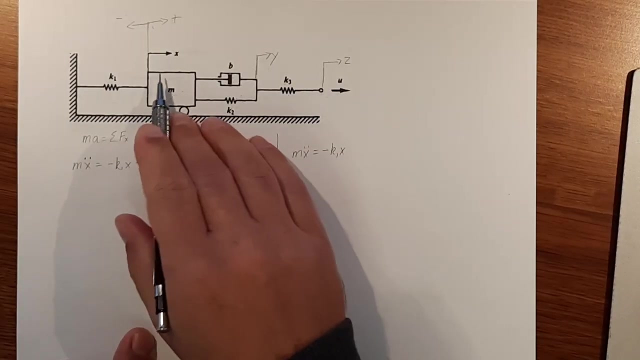 to write more equations to account for each section and its movement. And now for the second way to do. it is: we can have our mass times. acceleration is equal to our k1.. So minus k1, x, and now we have our dampener and spring. 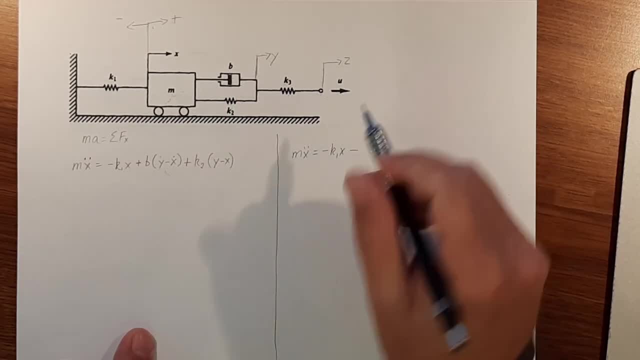 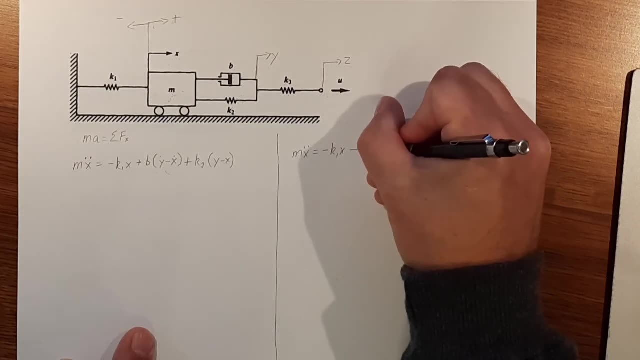 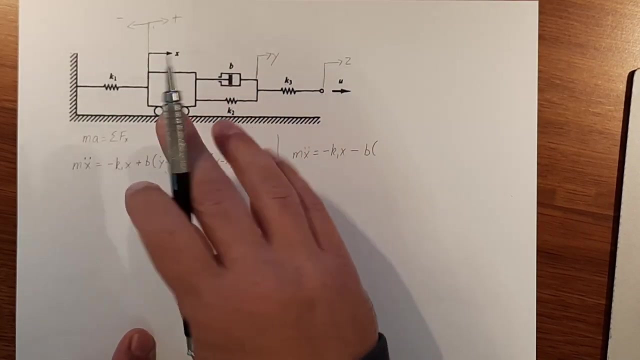 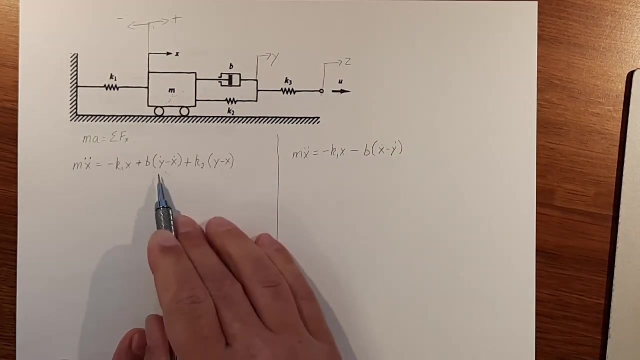 So if we want to keep the consistency of just subtracting everything, we can subtract b, but when we do the change in position to account for that, we have to flip the x and the y. So now we're going to have x dot minus y dot, instead of the y dot minus x dot, And then we have 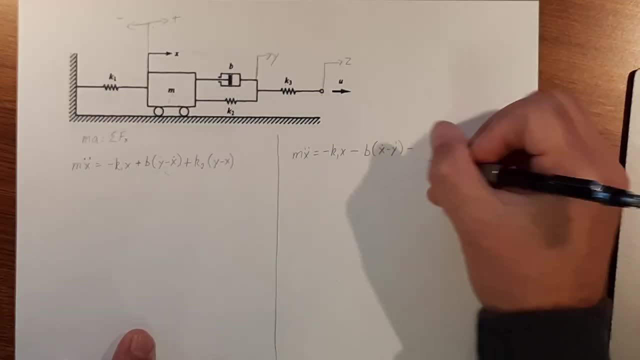 ourрастime divided by sweat over x, divided by thin pressure. OK, so what we have now to do is we're going to have to divide the k2, so we'll subtract it. We get k2 times again. we have to flip the y minus x. 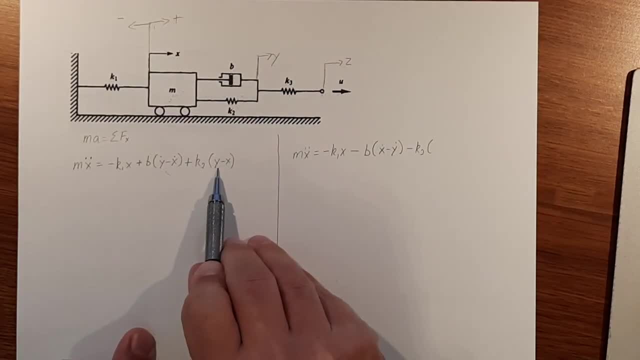 so we have x minus y, All right, so we have both different ways that we can write this. So let's go on and find our second equation. so we'll look at left over grand 8 and then we'll draw the y second equation. 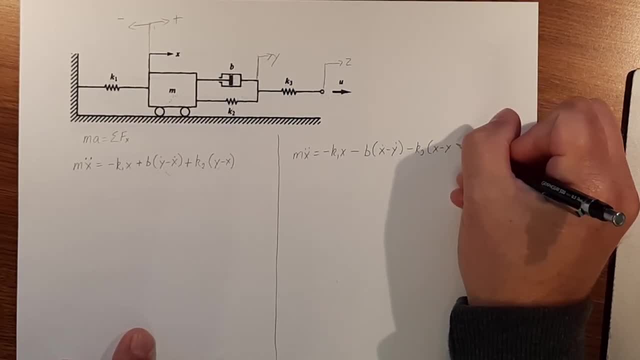 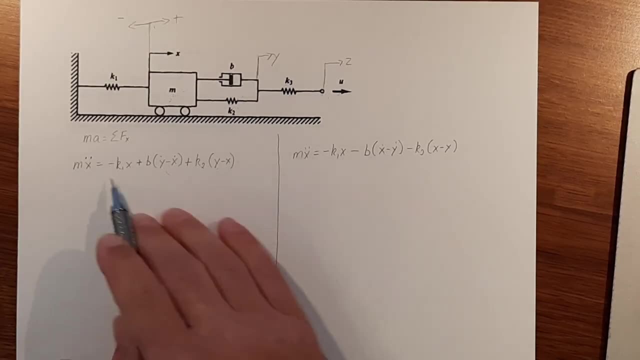 But let's look atnee way of this equation. so we have something to do with. that's right Now. if we want to solve this, it's just going to have to start that first formula, and here's an example of what this one looks like. 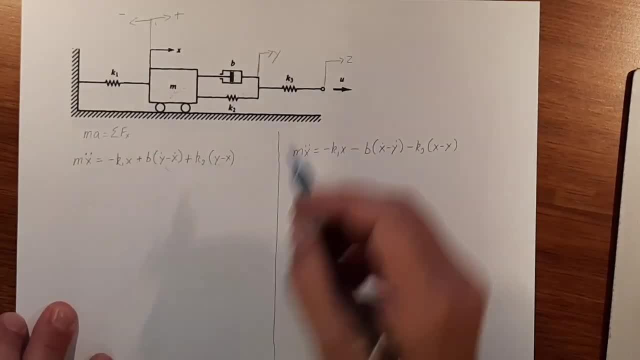 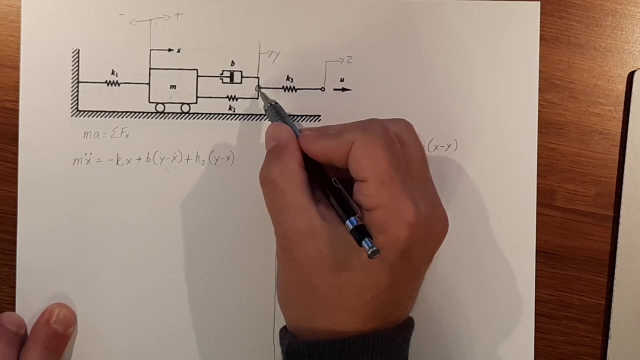 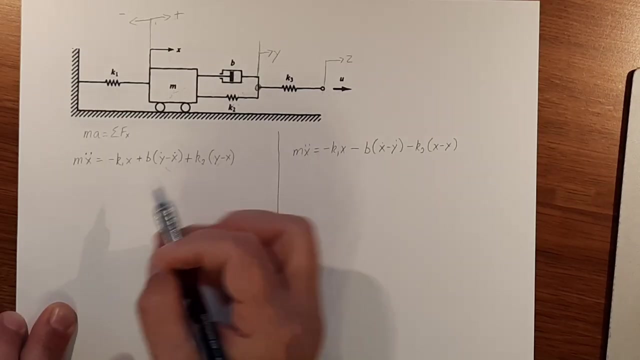 so let's go on and find our second equation. so we're going to be looking at this point in the system. so we want to know how this side affects this side. so if we look here, we do, the sum of forces are equal to zero, because this force has to equal this force for this to move. 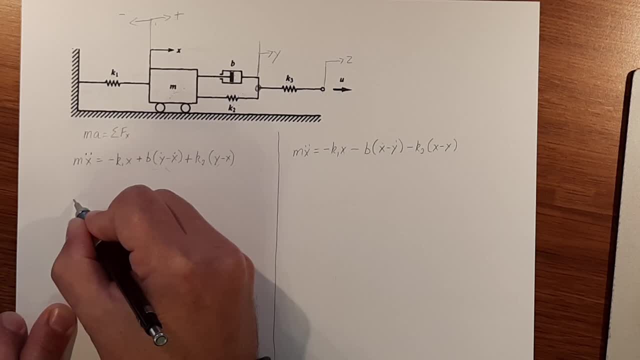 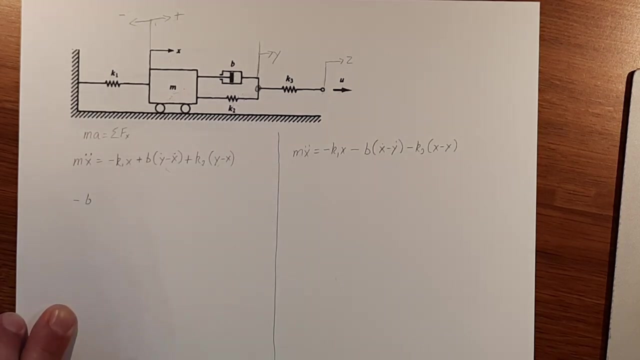 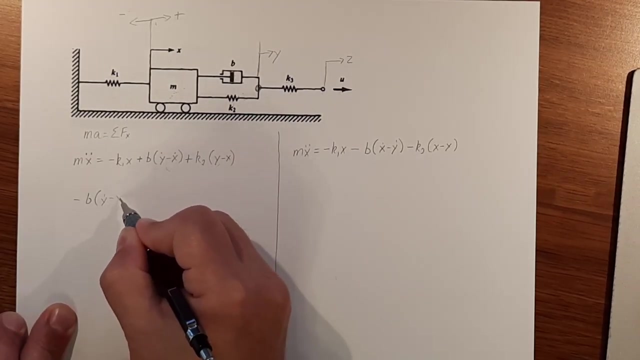 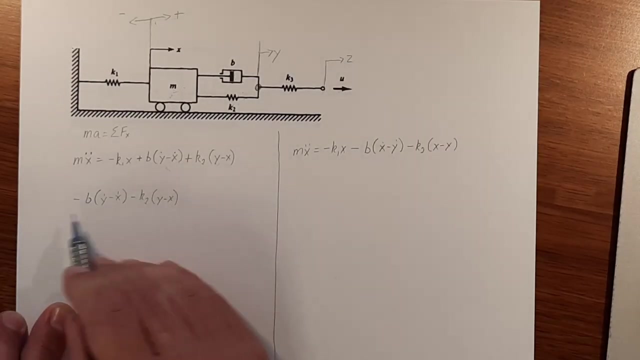 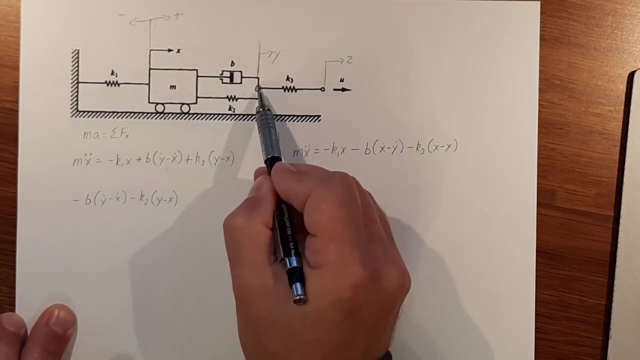 so we'll have a mine. so we'll have a minus b times its change of position, which is y dot minus x dot, and a minus k2 times its change in position, which is y minus x. now these are being subtracted because they are directly on the left side of this point, and that is going to equal. 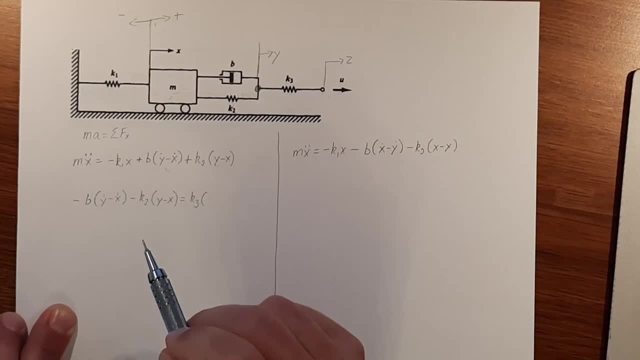 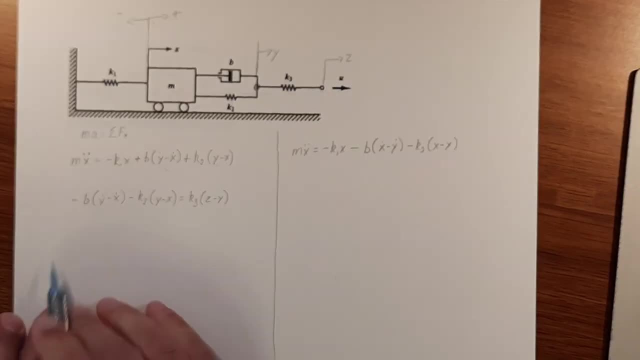 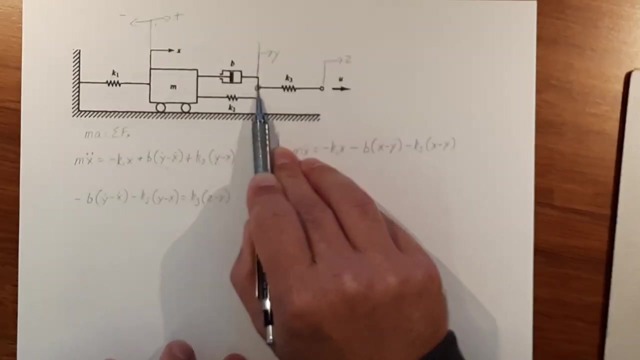 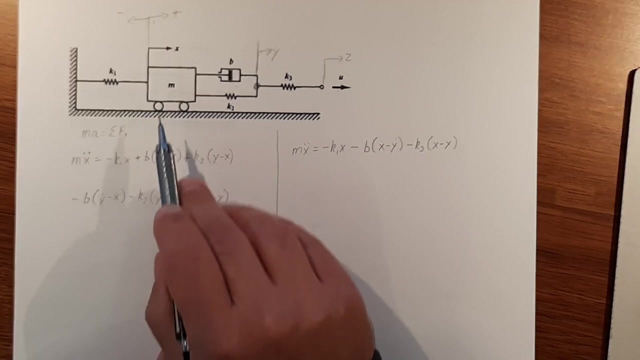 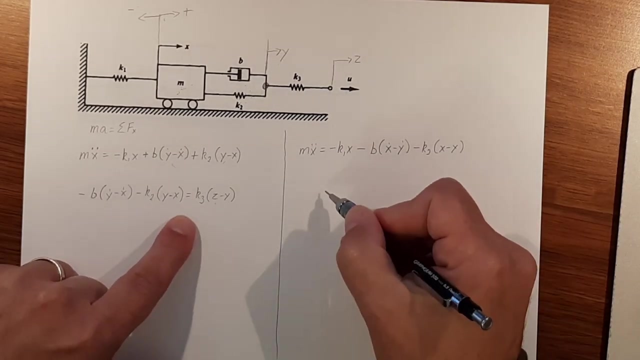 k3 times its change in position, which is c minus y. so the reason we write it this way is, like i said, is we need to look at this point here and understand that these two forces must be equal to be able to move the mass. so that's why we're making them equal. so on this side we can write this: 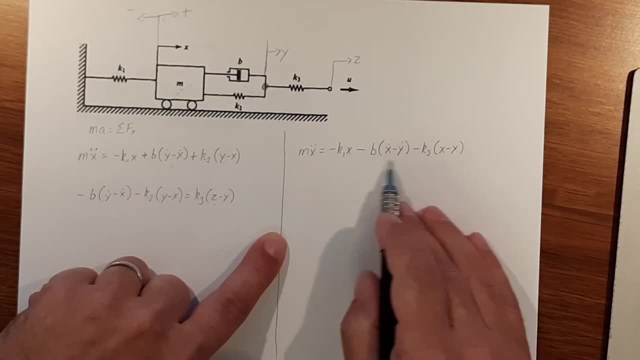 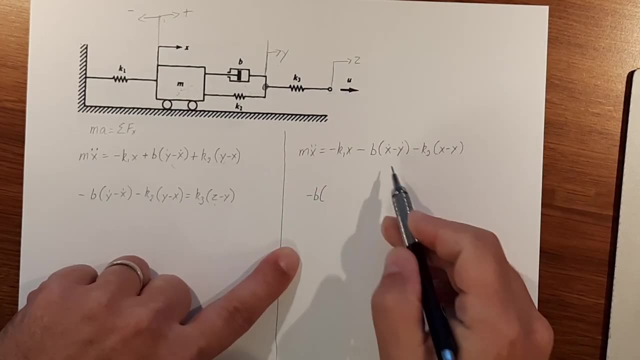 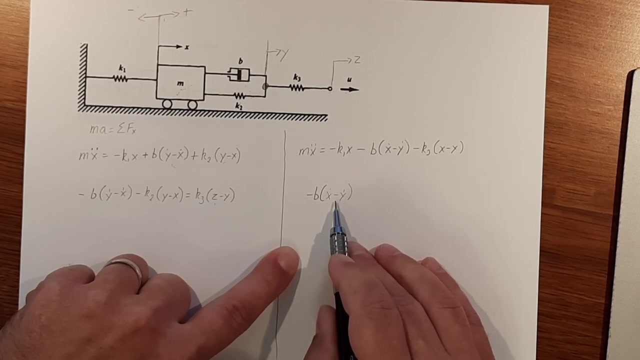 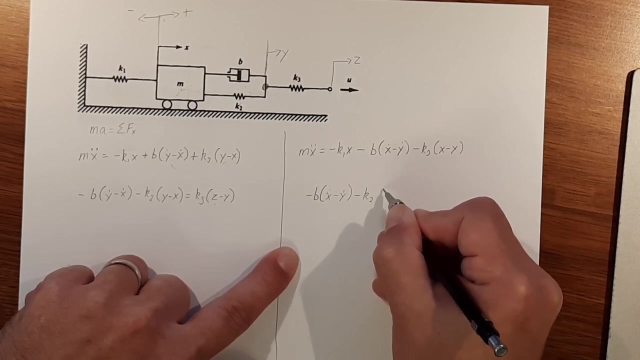 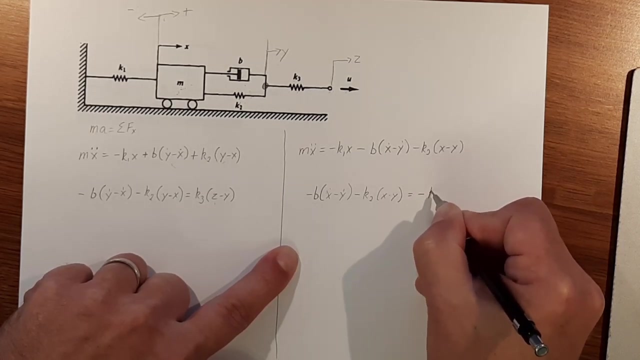 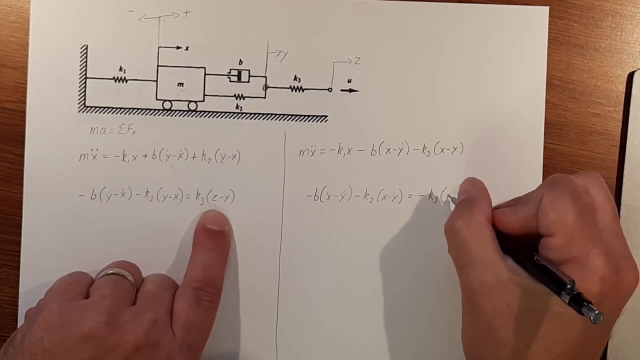 as keeping the normal subtracting. everything is again minus b, and again we have the x dot minus y dot, because we have to flip it: minus k2, x minus y and that's going to be equal to minus k3. and here we have to flip on this side to a y minus z. 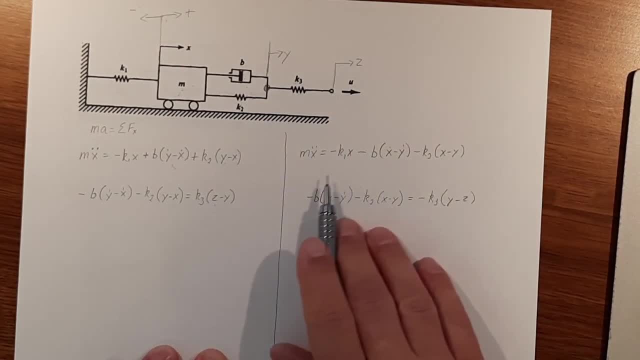 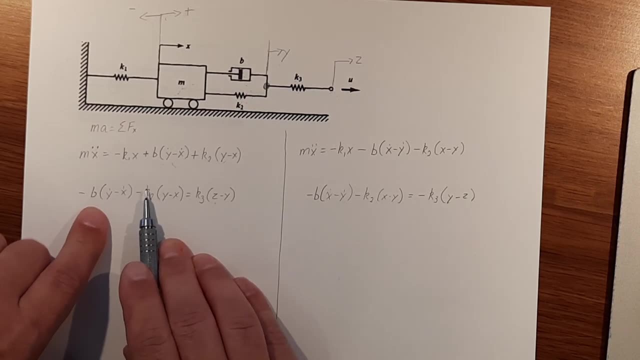 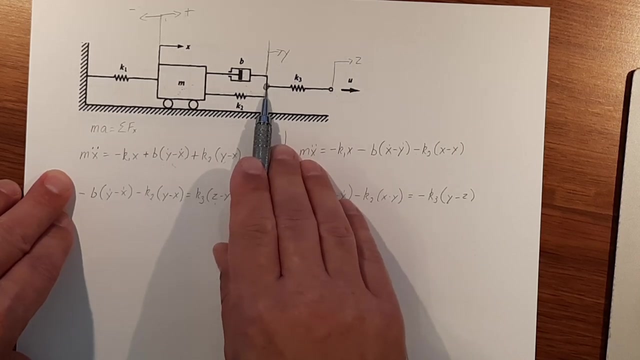 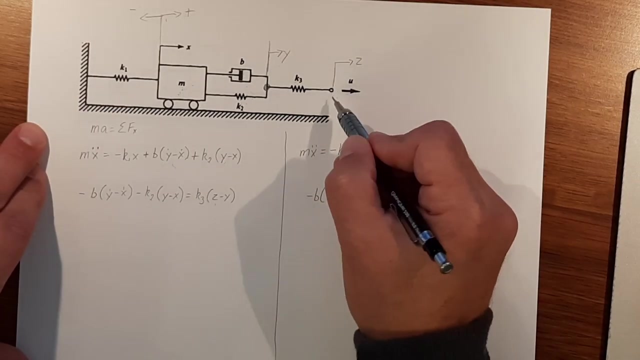 so one side, we try to keep everything as being subtracted from this mass and its acceleration and on this side, we're writing it out as the forces on each single point and how they react. so now for our third equation is we're going to be looking at this point? 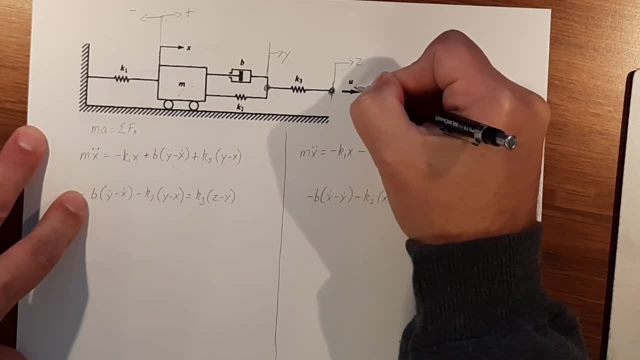 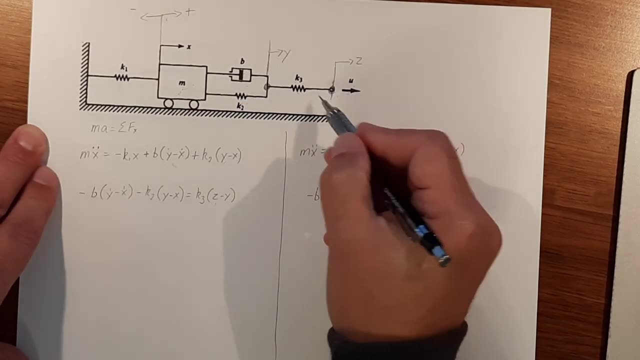 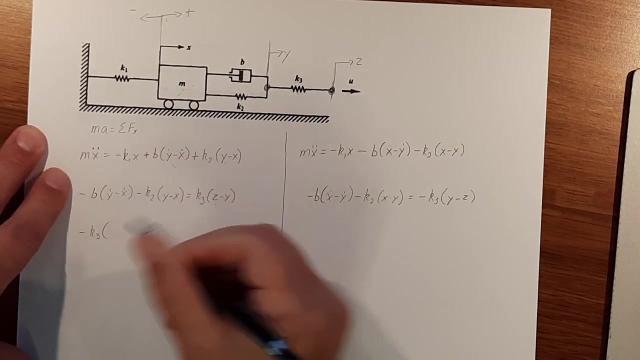 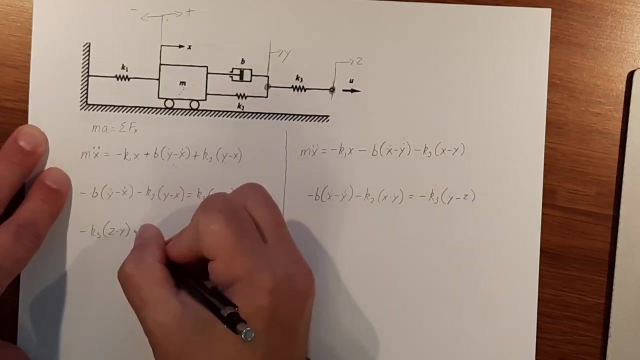 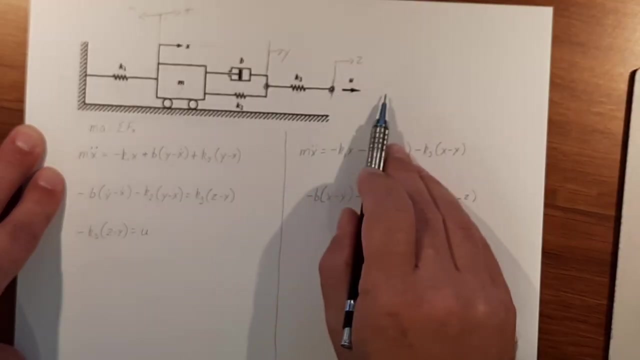 so here we're looking at how u is represented by k3. so k3 is on the left, so we're going to subtract k3 and our change of position is z minus y and that is going to be equal to. u now use positive because it's pulling it to the positive. 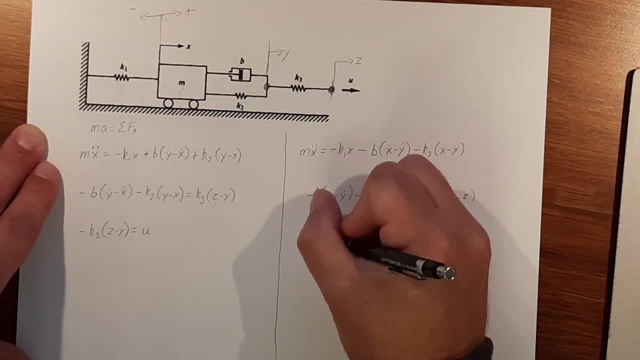 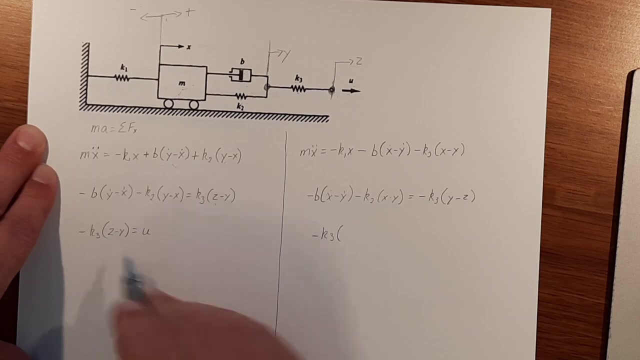 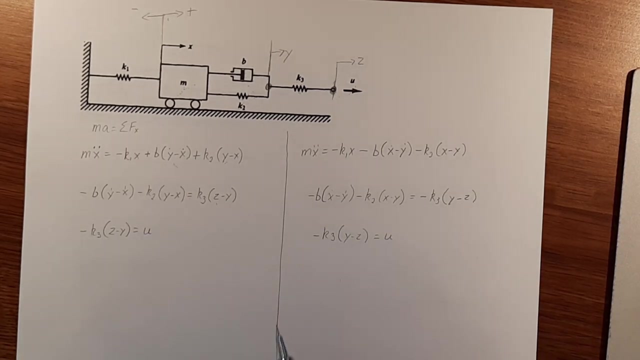 side, and on the side where we're trying to keep everything negative, we're going to have that minus k3 and we're going to flip that again. is y minus z is equal to u. now u is going to stay positive because u is a positive force. 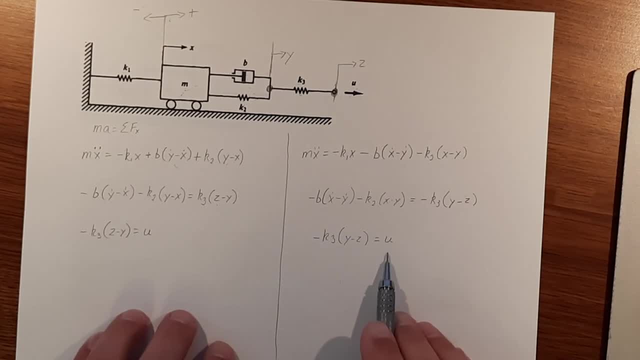 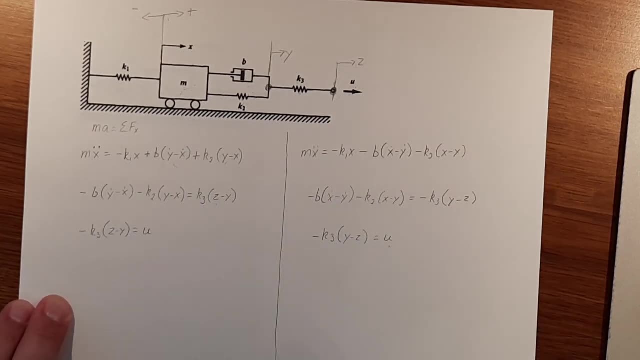 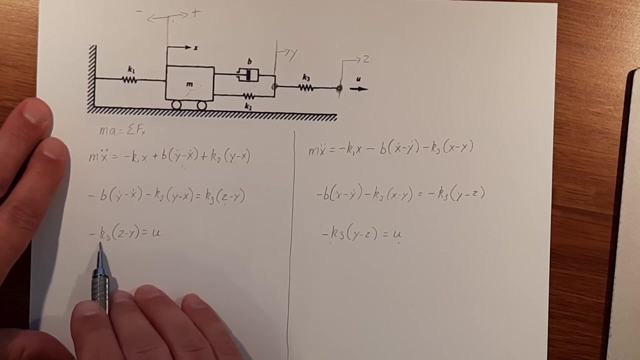 and we know that the input has to be positive. so u is going to stay positive. but now that we have our three equations, now we can start rearranging, substituting back in to the other equations. so if we look here we have that, let's start over here. so we have a minus K 3 times Z. minus Y is equal to U. 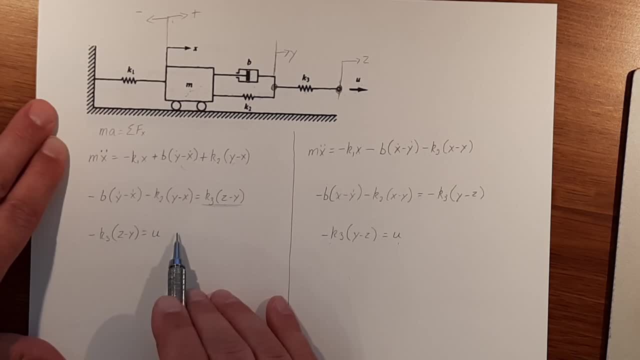 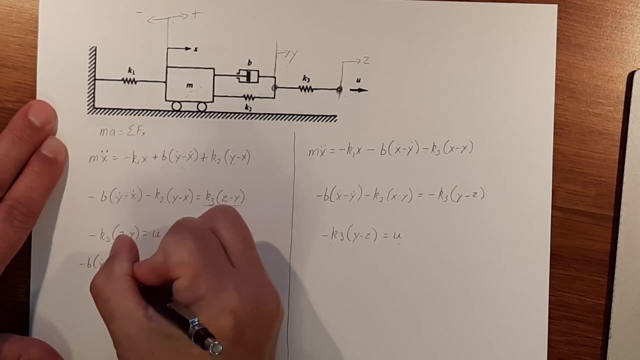 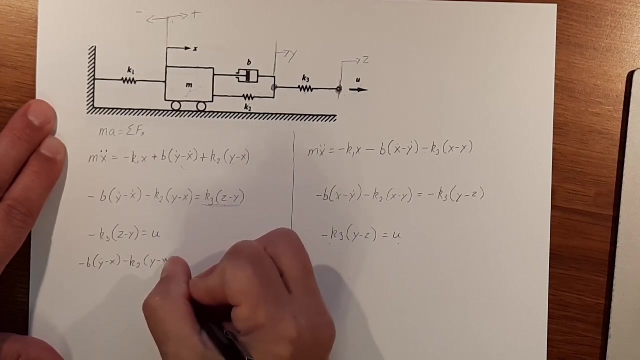 and we have a K 3 Z minus Y here. so what we're going to do is we're going to substitute that minus B, Y dot minus X minus K. 2 Y minus X is equal to, since we have a minus K 3 times Z minus Y here. we're going to keep the negative and 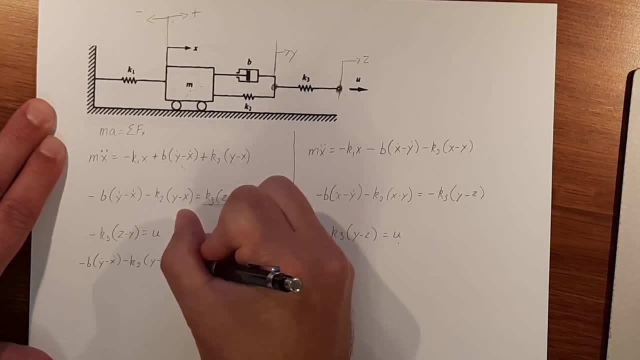 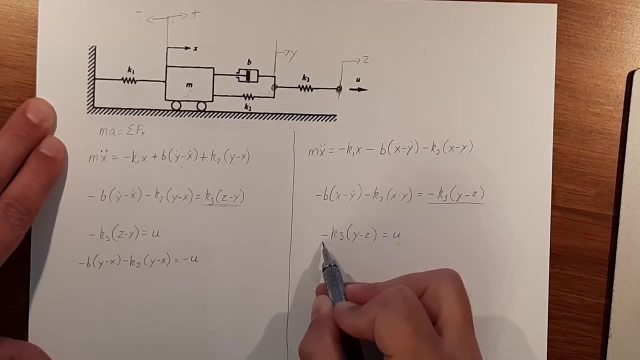 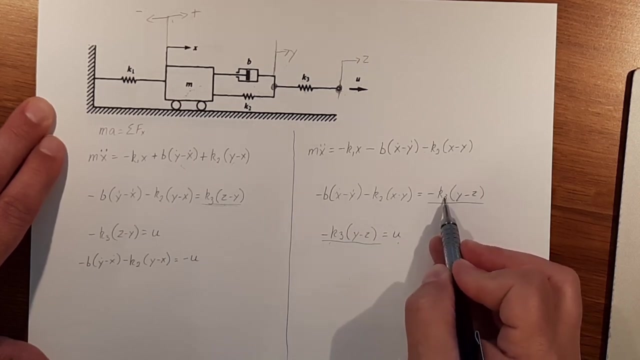 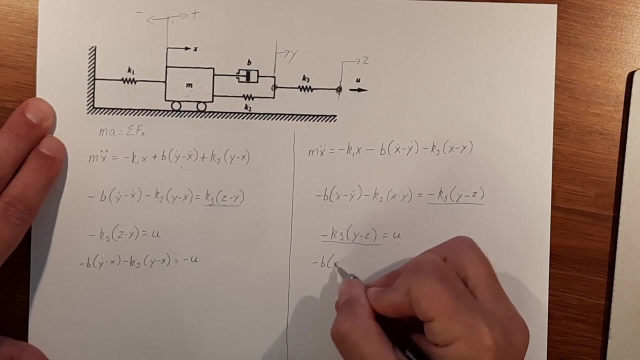 have that it is equal to a negative U. so on this side we can can substitute. since we have negative k3 times z minus y is equal to u. we can just directly substitute k3 y minus z in. So we're going to have a minus b, x, dot minus y, dot minus k2 x. 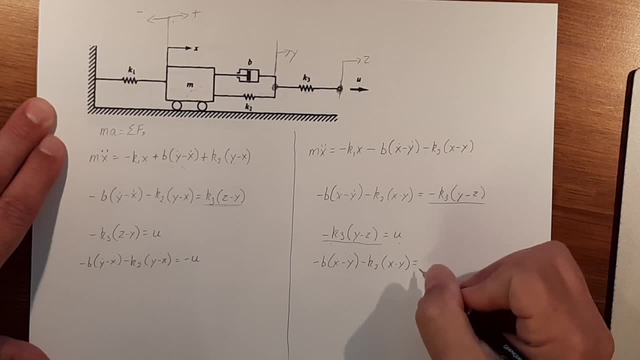 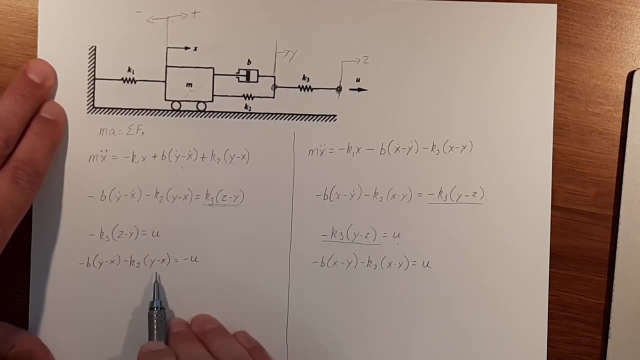 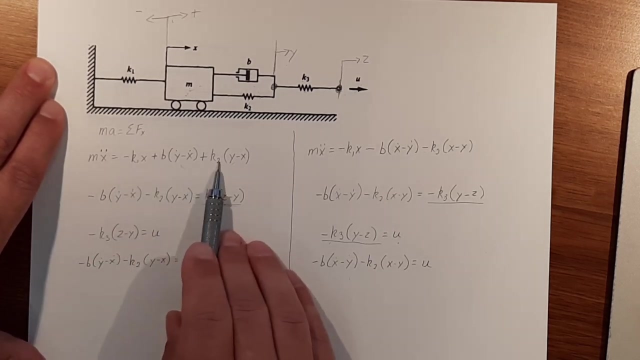 minus y is equal to direct substitution. is u All right? so now we look at this equation and how we can substitute it into our first one. So we have a plus b and a plus k in our first one, but over here we have a minus b and a minus k. 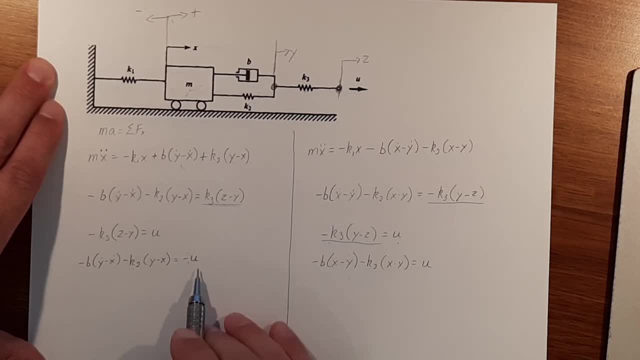 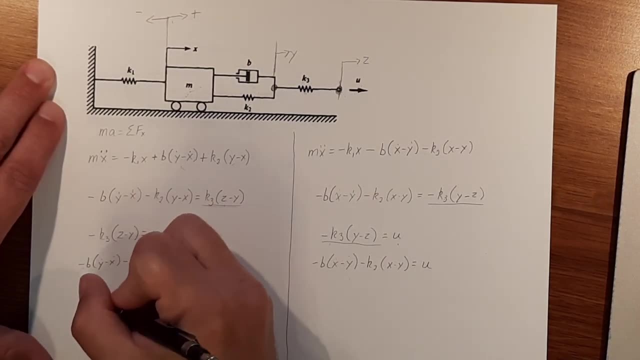 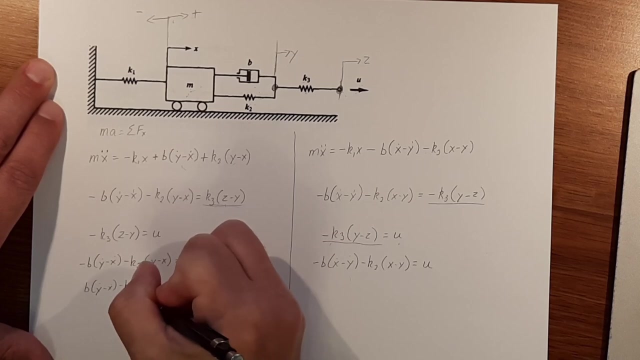 But we also have minus u, so we could either rearrange or multiply the whole thing by a negative one, which would give us a b y minus u. So we have a minus b, y minus x, dot minus k2. y minus x is equal to u. 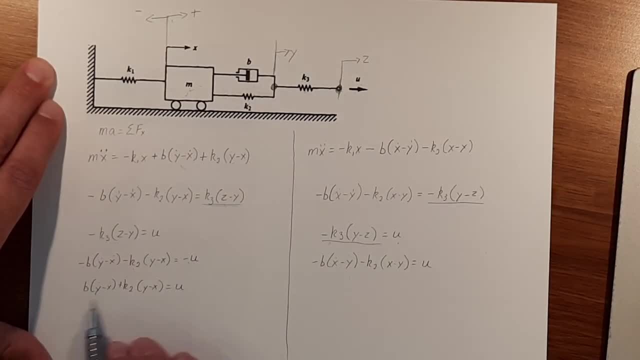 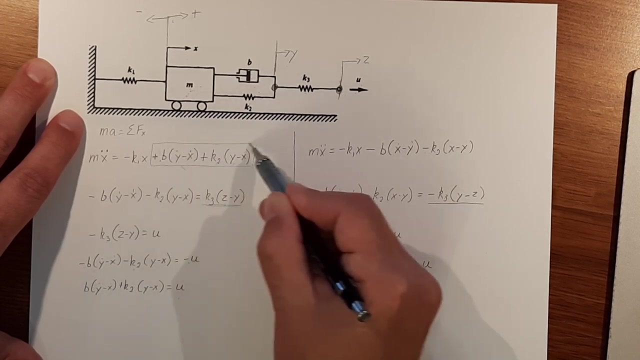 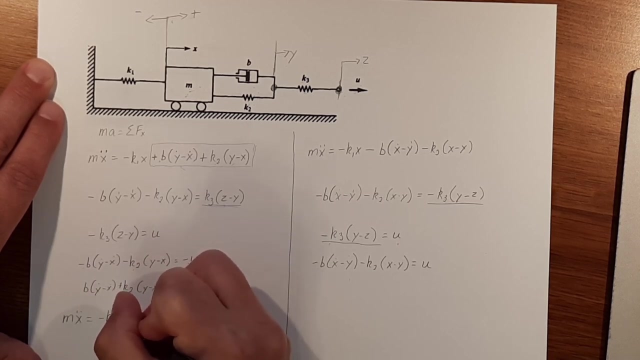 Now a plus, So we have a b plus k equals u. Now we can match up here, because we have a plus b plus k, So this now can all become u. So then we have m x double dot equals minus k1, x plus, substituting that in u.